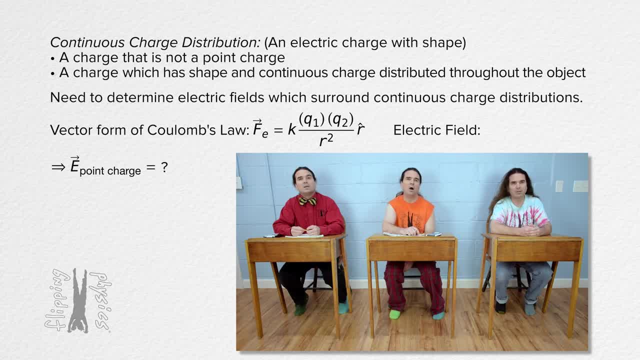 of charge of the two charges all times unit vector r. The equation definition of the electric field is: electric field equals electrostatic force divided by charge. where both electric field and electrostatic force are vectors, That means the electric field caused by a point charge. 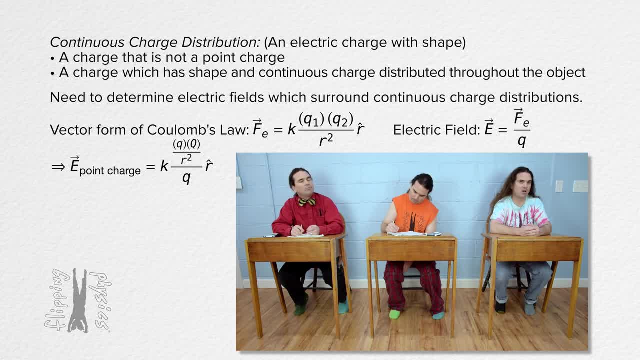 equals the Coulomb constant times the charge of the small positive test charge. little q times the charge of the point charge. big Q divided by r, squared all divided by little q, and then all times unit vector r Little q. the charge on the small positive test charge. 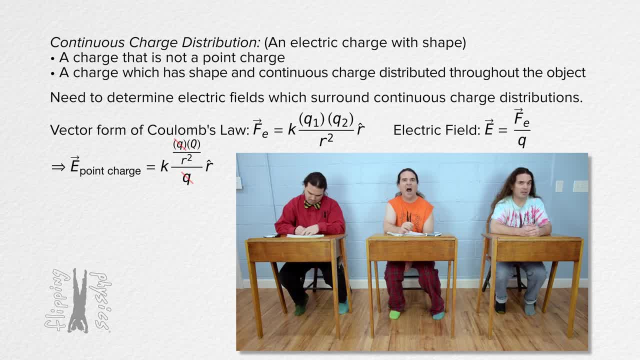 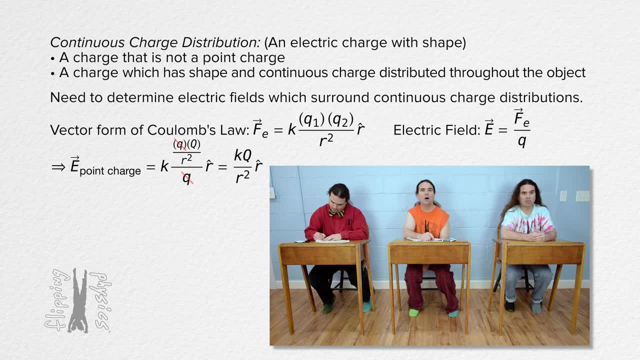 cancels out and we get that. the equation for the electric field which surrounds and is caused by a point charge equals the Coulomb constant times: the charge of the point charge divided by the square of r, the distance between the center of the point charge and the location where we are. 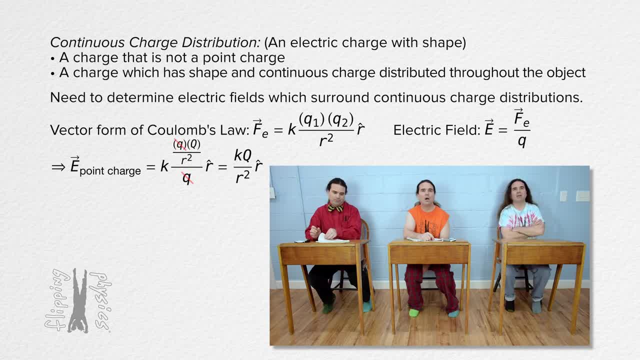 defining the electric field all times, unit, vector r. But I still don't get what this has to do with the electric field caused by a continuous charge distribution. Thank you, Bo. Hopefully what I'm about to say will clear up a little bit of your questions. I'm going to go ahead and wrap this up. 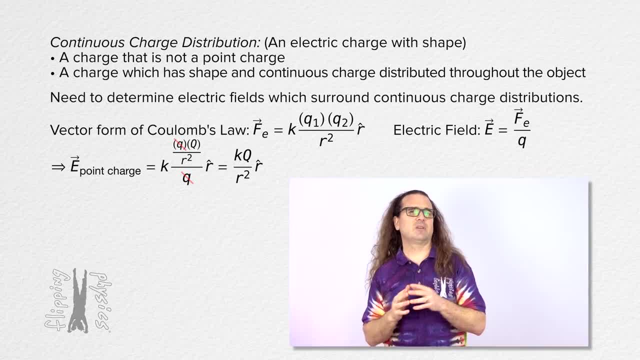 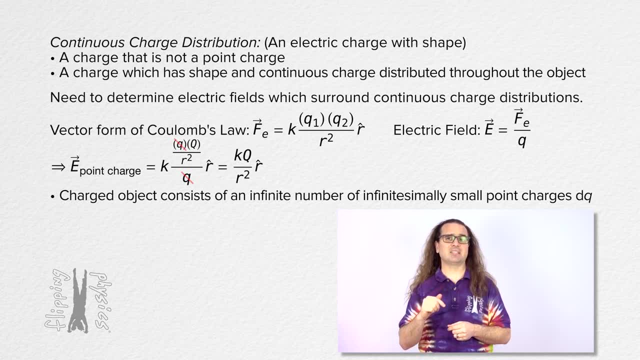 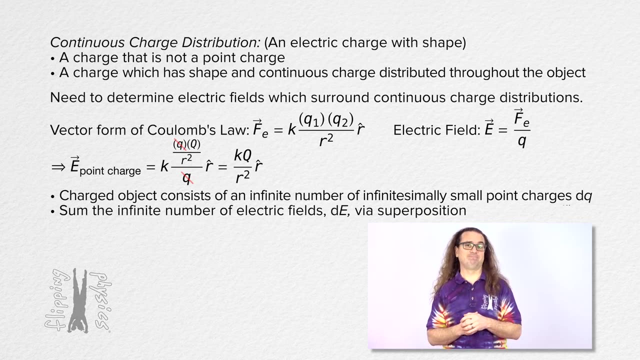 and I'll see you in the next video. Let's clear up those doubts. We're going to consider the charged object to be made up of an infinite number of infinitesimally small point charges, dq, and add up the infinite number of electric fields via superposition, It's an integral. 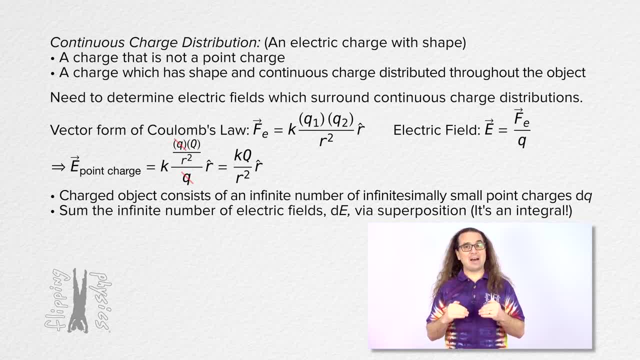 Oh Yeah, Okay, Exactly, We now know dE, the electric field caused by every infinitesimally small part of the continuous charge distribution. dq equals the Coulomb constant times dq divided by r squared times, unit vector r. We can take the integral of both sides, which adds up the: 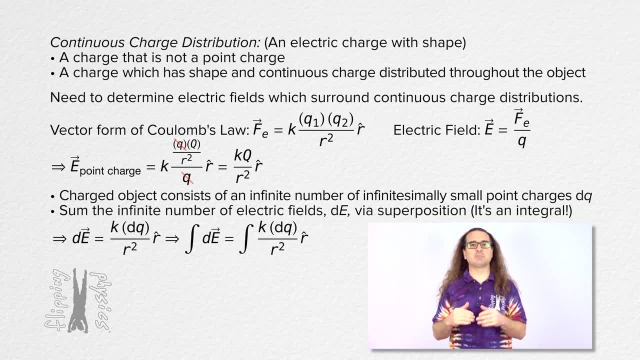 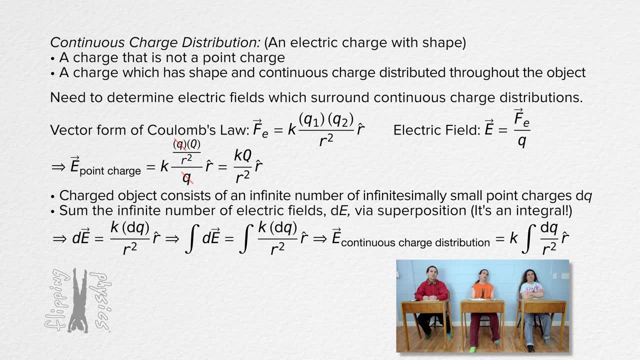 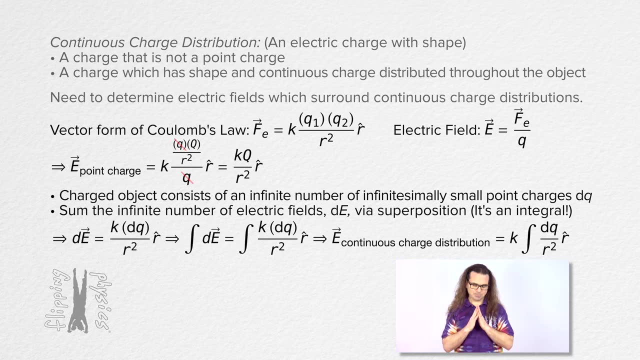 electric fields caused by the infinite number of infinitesimally small point charges, dq, and we get the electric field caused by the continuous charge. distribution equals the Coulomb constant times, the integral of dq over r squared all times, unit vector r. Okay, Bobby, please review the three charge densities. 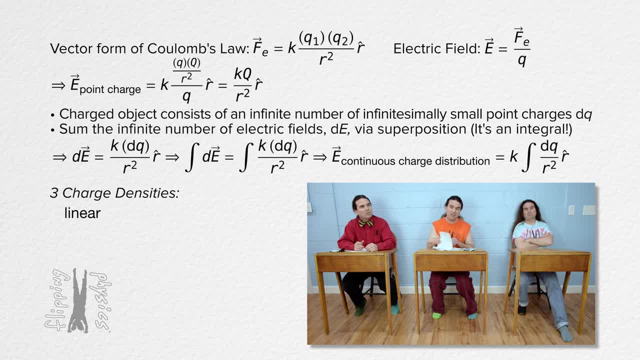 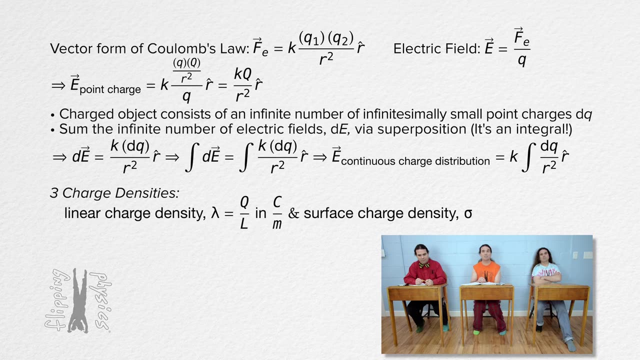 Sure Linear charge: density or lowercase lambda, equals charge divided by length, so it's in units of coulombs per meter. Surface charge: density or lowercase sigma equals charge divided by area, and the units are coulombs per meter squared. 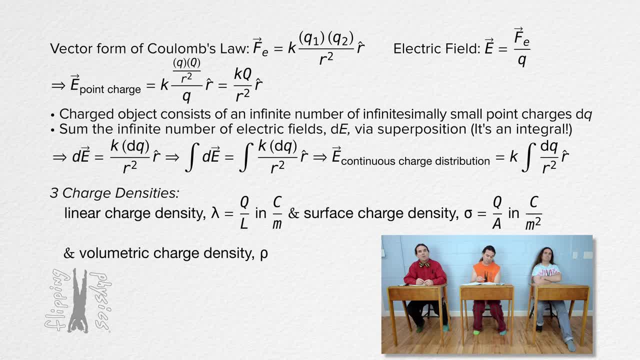 And volumetric charge. density, or lowercase rho, equals charge divided by volume, and its units are coulombs per meter cubed. Great. Thank you very much for learning with me today. I enjoy learning with you. 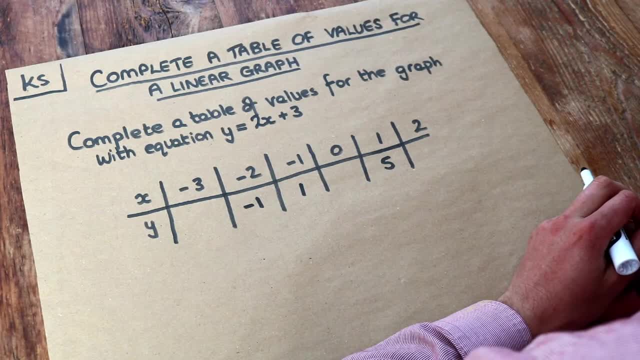 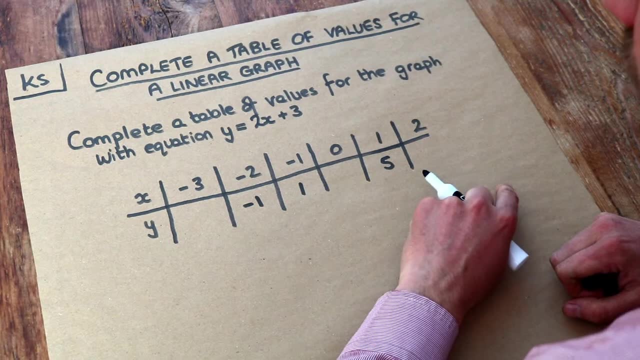 Hello and welcome to this DrosMaths key skill video on completing a table of values for a linear graph. So we've got different values of x minus 3, minus 2, minus 1, etc. And we want to work out the y values for each of those x values. 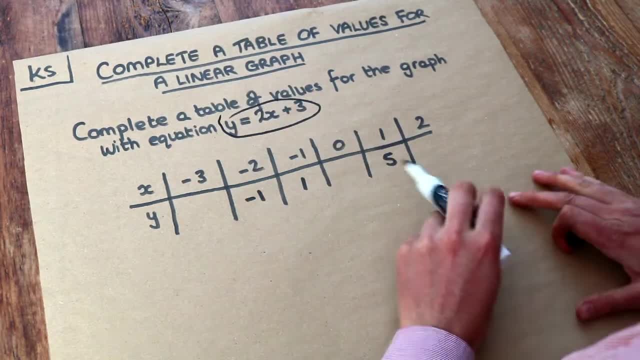 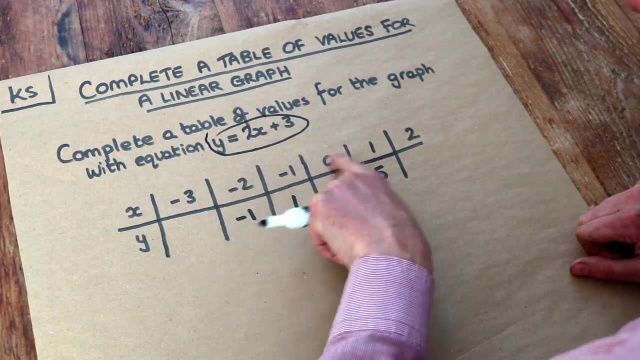 And we're going to use this equation here as like a rule for telling us how do we work out the y value based on the x value, And basically, all we need to do is to take each of these values of x and substitute it into this equation. 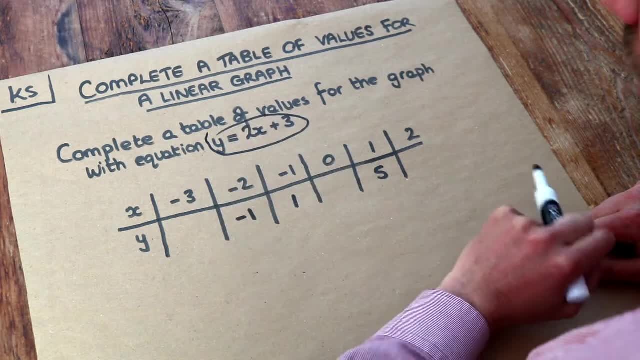 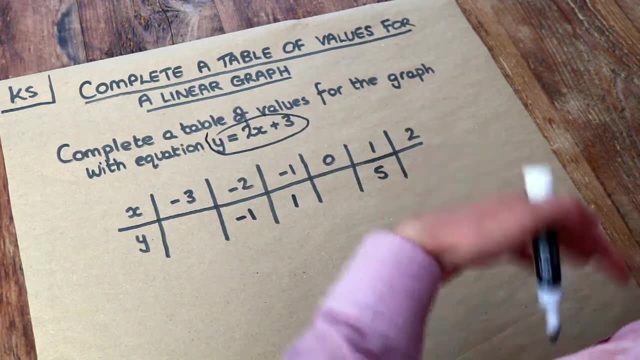 And that allows us to work out what the y would be for particular values of x. And if you're wondering what's the point of doing this, it's because usually you would then take this table of values and you would plot that as a graph.